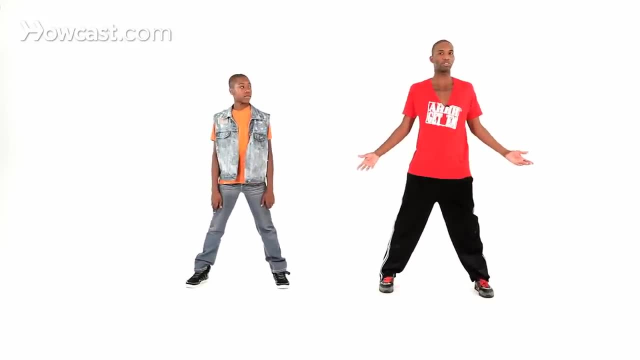 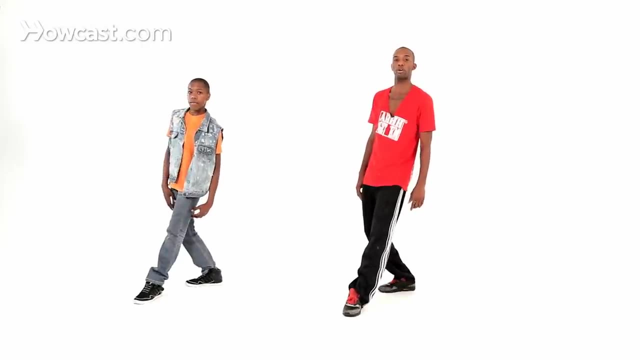 Then I go the other direction. Three, One, two, three, You got that part, Yeah. So now I'm going to take my left and go diagonal and there I have four. Bring this one behind five and then I'm going to jump. 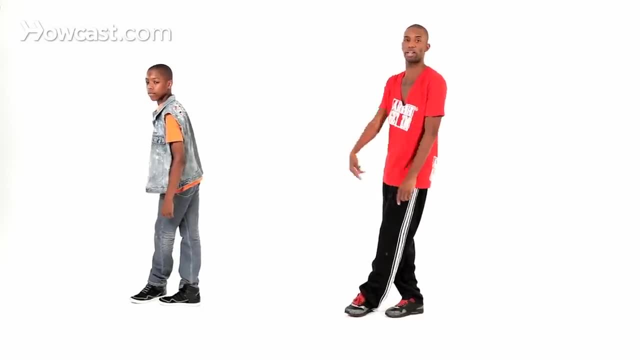 And I'm going to take my right foot, which is now in the back, and bring it up in the front and I'm going to have six, Six Throughout the whole thing. I hope you're noticing that it's right, left, right left. 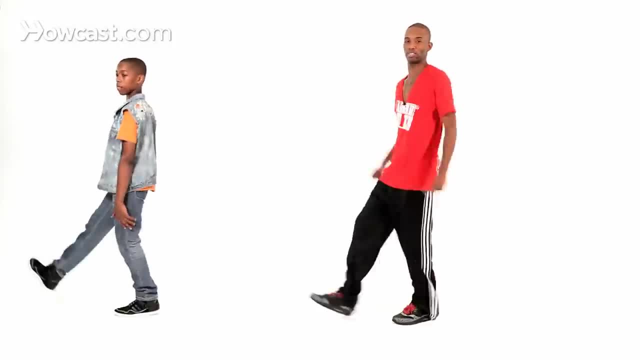 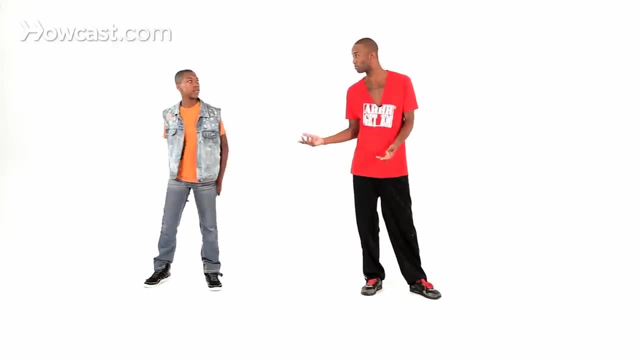 right, left, right switch Got it Just like walking down the street Right, left, right, left, So you're never going to do the same foot at the same time. It'll work out for you. Let's try it again. 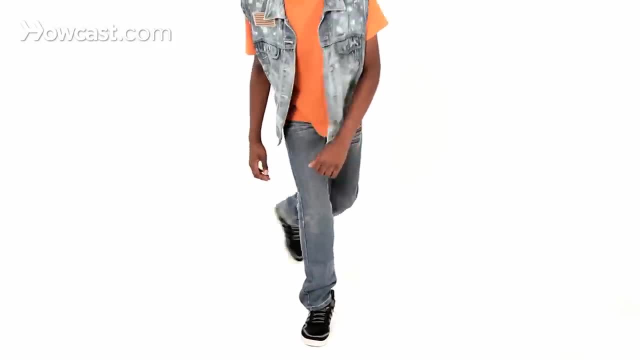 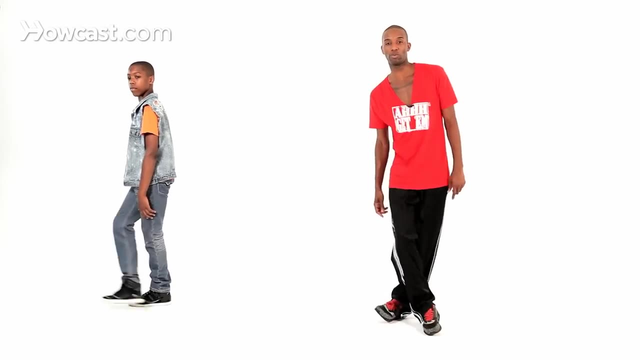 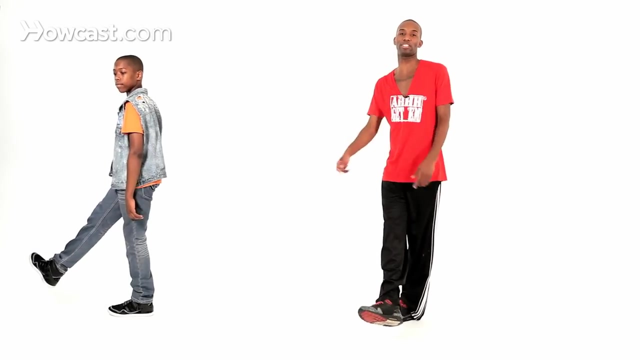 Swing the right leg around. You're going to go: one corner, two corner, three, four, five, six. Repeat: One, two, three, four, five, Six. There's your six step. We're going to take it down to the floor because you do a six step down here anyway. 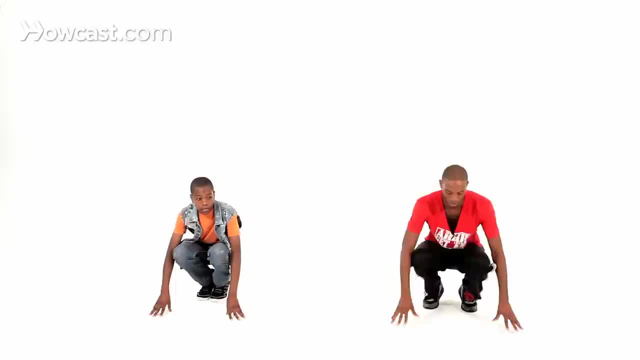 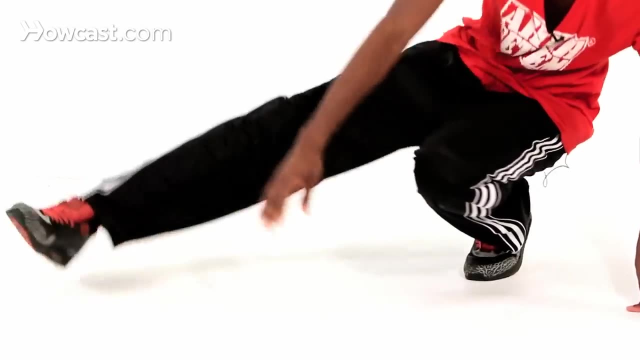 And my heels are off the floor, so I'm like this right. So you're in this position. You're going to take your right leg, stretch it out knee straight and bring it all the way around to the front. There's your one. 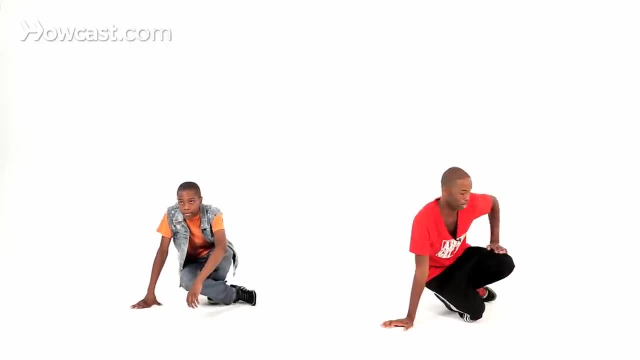 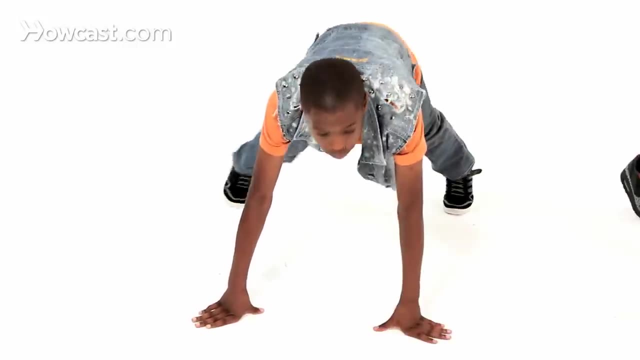 That's the circle I was talking about. Now I'm going to step to the back corner with my left foot and there's going to be my two. So I go two, I take the other leg and I go two. I take the other leg and I go three. 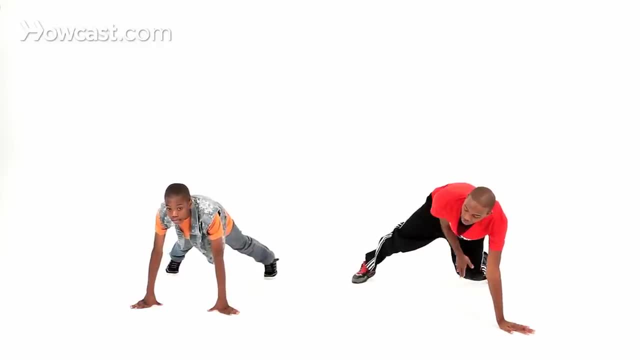 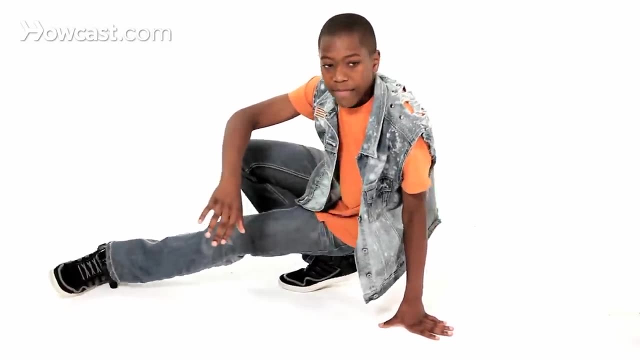 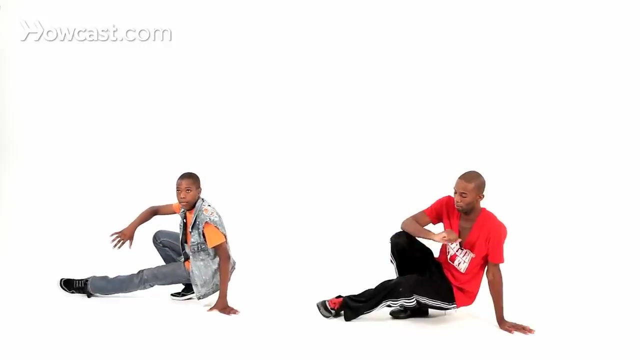 Now I take my left and I bring it diagonal across and I got four. See that I take my right foot five. From here, the jump switch that you did earlier is going to happen on the floor. Might feel a little bit weird to you, but I'm going to do it now without using the hands. 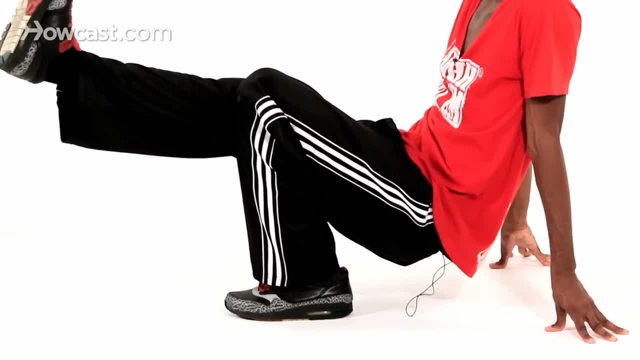 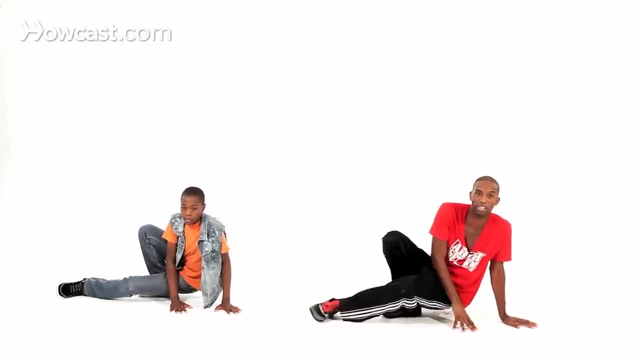 so you can just see what it looks like. Basically it's like this. Now, going back to where I was, I had my hands on this side, So I'm going to jump and bring my hands to the other side. It looks like this: 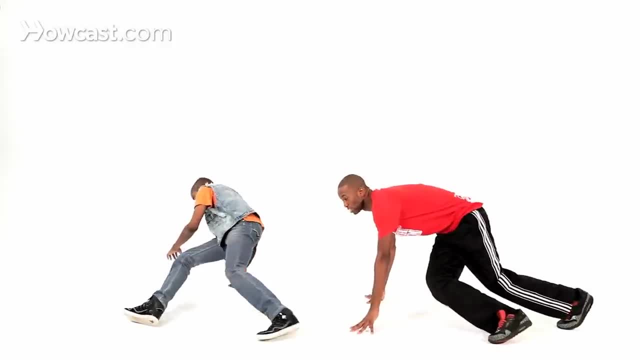 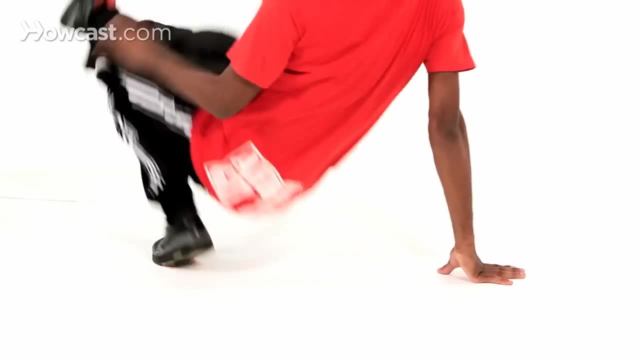 There you go, Got it. Now step to the corner. Step to the corner again, Step diagonal. Bring it in. Then I do that jump. There you go. All right, We're going to try it from the beginning One more time. nice and slow.